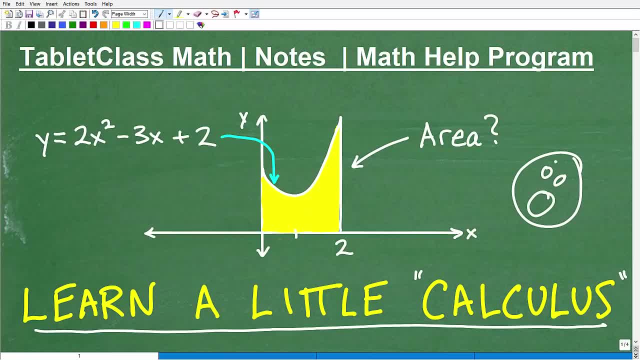 They're like calculus- I've heard of that, It's that scary math, you know- And they're like, oh no, calculus, it's very, very difficult. It's almost like some sort of torture or whatnot. You know, like I'm going to assign you, maybe you did something wrong. 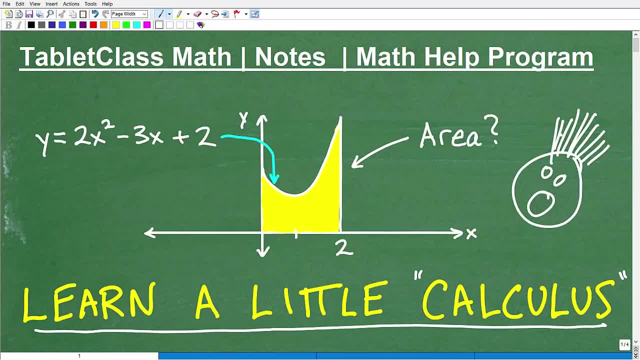 and you were sentenced to 10 years hard time by taking 10 years of calculus. I don't know. I think sometimes people think of math in general as some sort of torture. But listen, we've got to relax about this stuff. And calculus it is an advanced math. I'm not going to try to say it isn't. 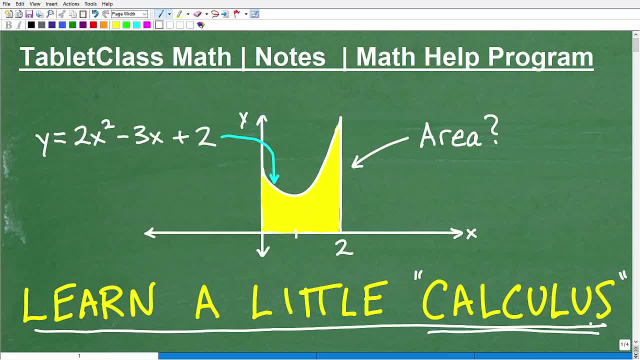 But you can definitely understand the essence of it with some basic problems like the one I'm going to show you here. So I'm going to demonstrate a little calculus here. We're going to solve this problem. Now, what is the problem? So you can see this little yellow shape right here, this crazy shape. 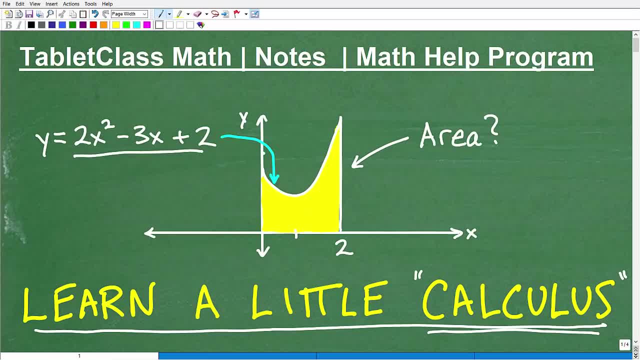 And it's defined by this function, okay, And it kind of borders the y-axis and the x-axis And we want to find the area of that nice little yellow shape. Now you're like: oh, area. Yeah, well, if I had a triangle and I was trying to figure out the area of that thing. 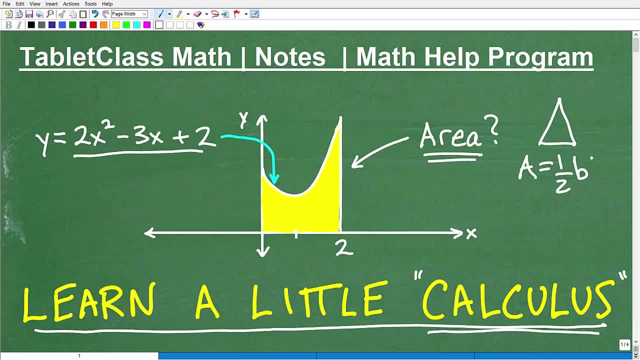 I could just go. oh yeah, area equals one half base times height. Well, if I had a circle, I could go. area equals pi r squared. If I had a rectangle, I could go. area is equal to the width times the length. 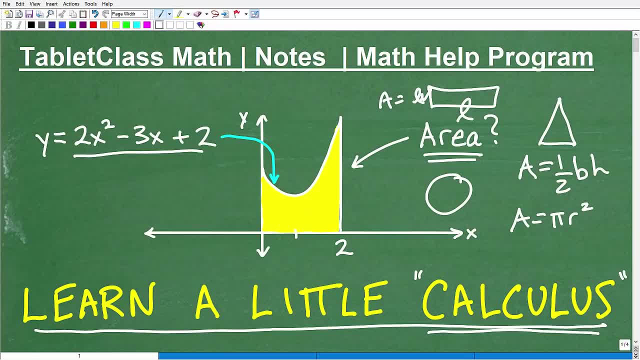 You kind of get the idea if I had a trapezoid, et cetera, But guess what? We don't have a handy-dandy formula for this crazy-looking shape that we're dealing with right here. Okay, So the only way we can get the area for this guy is to use calculus. all right, 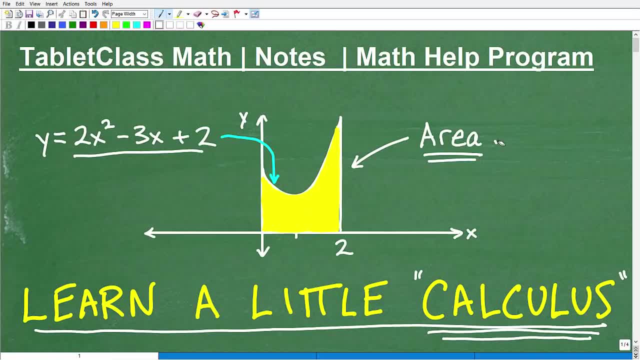 So this is one of the, you know, key things that we do in calculus. It's called integration. We use this crazy-looking, mysterious symbol like that. So I'm going to actually show you this here, And it's going to take all of about a couple minutes to actually calculate the area of this thing. 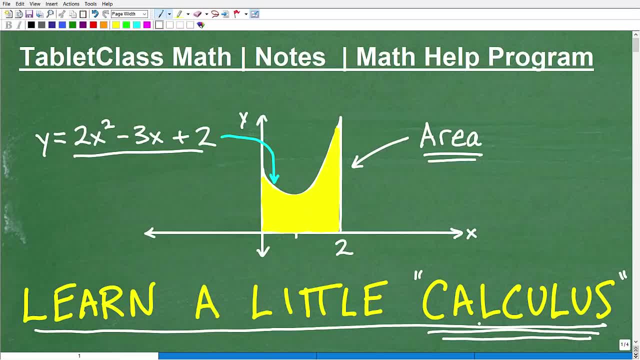 So if you're interested in seeing how calculus works- you know basic calculus. well, let's stick around, okay? So again, even if you only have a basic math level, don't feel like this is going to be beyond anything. 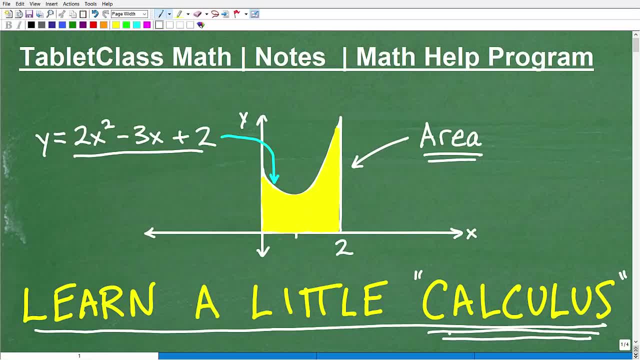 You can't understand, okay. So I'm going to do my best to get you motivated about the subject of calculus. But first let me quickly introduce myself. My name is John. I'm the founder of Tablet Class Math. I'm also a middle and high school math teacher. 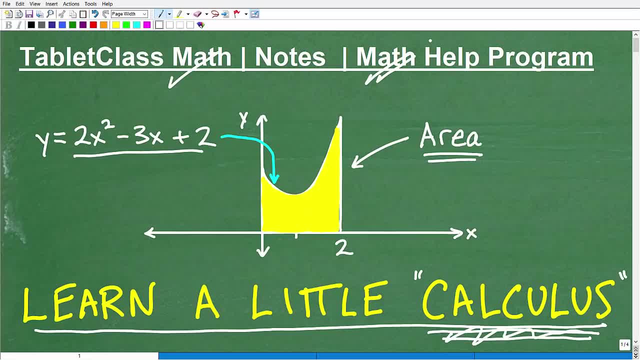 And over several years I've constructed what I like to believe is one of the best online math help programs there is. Of course, I'll let you be the judge of that. If you're interested, you can check out my math help program by following the link in the description of this video. 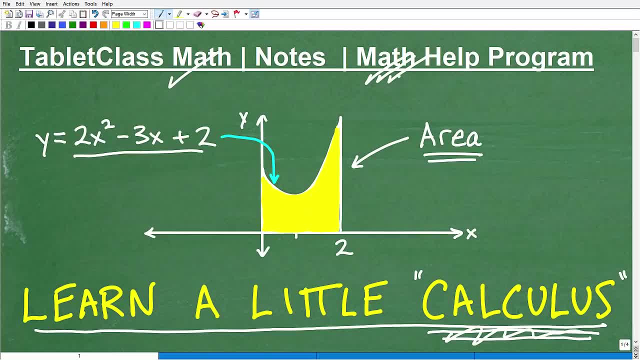 But basically I have 100-plus different math courses Ranging from pre-algebra, algebra and geometry, algebra 2.. I'm going to be launching pre-calculus here very shortly And pre-calculus very advanced mathematics, And this is all the stuff you need to have as a prerequisite in order to you know formally. take calculus: 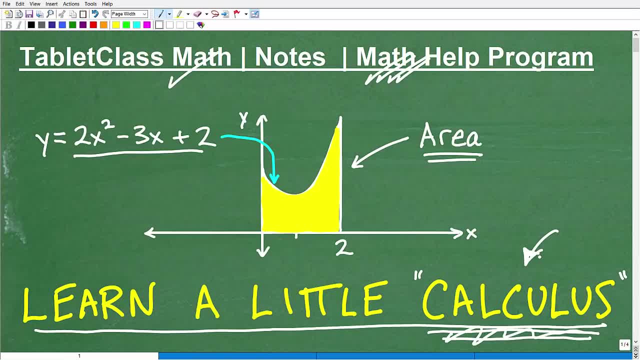 Because calculus it is. you know it is a sophisticated math, right, But there is some stuff that we can understand, that you know it's not overly complicated. So that's what we're going to be doing in this video. 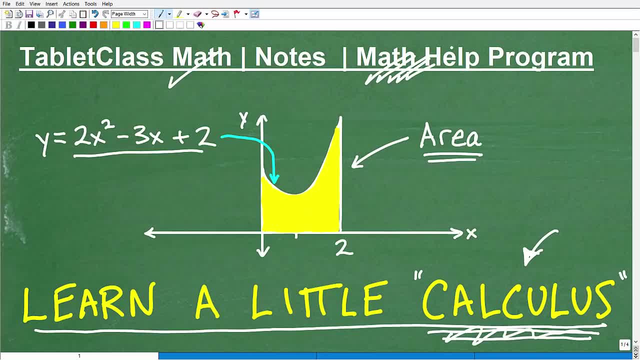 But I also do a lot of work In the area of test preparation. So if you're studying for an exam like the GED, HiSET, TASC, SAT, ACT, GRE, GMAT, ACCUPLACER, ALEX, CLEP exam, teacher certification exam and many others, 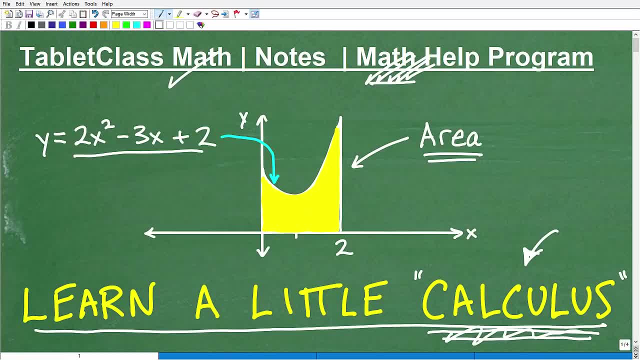 I can help you out prepare for the math section. Just go to my website, check out my full course catalog. If I do not have your exam, drop me a line and I'll help you out the best I can. I also do a lot of work with independent learners, like homeschoolers. 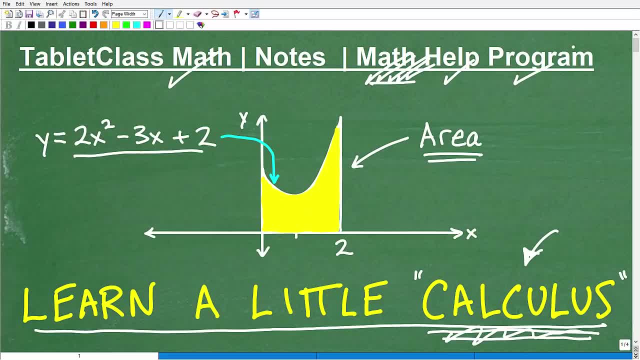 So if you homeschool, I have a great homeschool learning program, And then, obviously, I help those of you that are having a tough time- A tough time in your current math courses. Now, if you're truly serious about learning mathematics, whether you're a student or you want to take a math course, 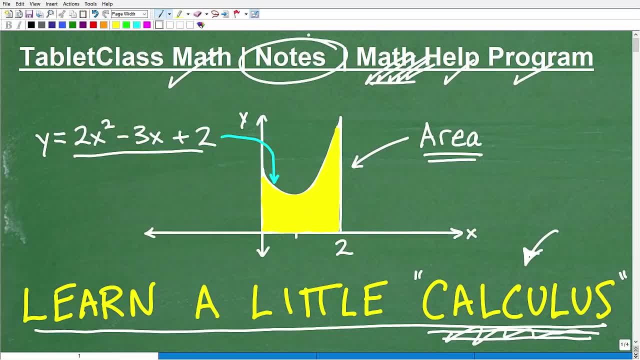 Then you've got to be serious about this. You've got to take great math notes. So I've been teaching mathematics for decades And it's apparent to me those students who take great math notes almost always get great math grades, And the reverse is true. 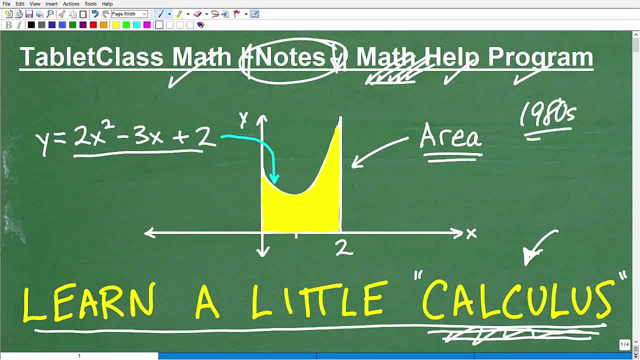 Those students were like me way back in the good old 1980s. That was almost too fun of a decade to grow in Because I was completely distracted And I certainly wasn't taking math notes. while I was writing notes But there were two of my friends saying: hey, what are we doing this weekend? 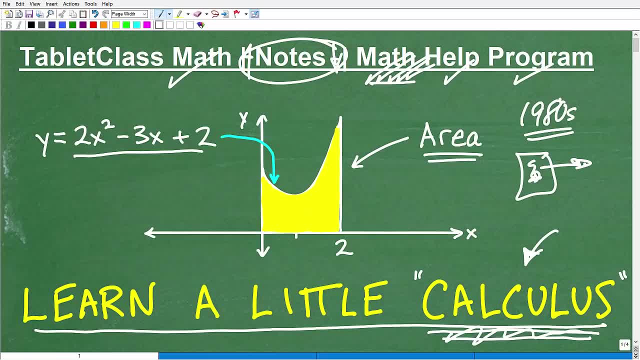 Okay, So listen, I've made all the mistakes and then some, But the bottom line is this: There's no shortcuts in learning. You have to be highly focused every single day or you'll miss too much. Okay, Start taking great math notes and you're going to see everything improve. 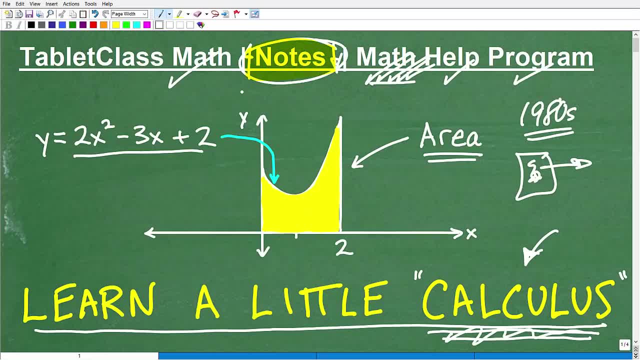 All right Now. in the meantime, you still need something to study from, So I offer detailed, comprehensive math notes that you can use. Those would include pre-algebra, algebra One, geometry, algebra two and trigonometry. You can find the links to my notes in the description of this video. 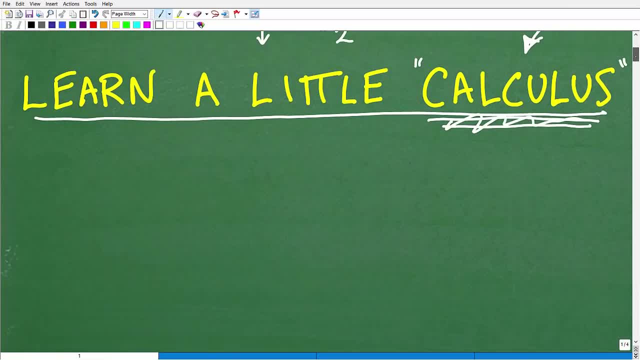 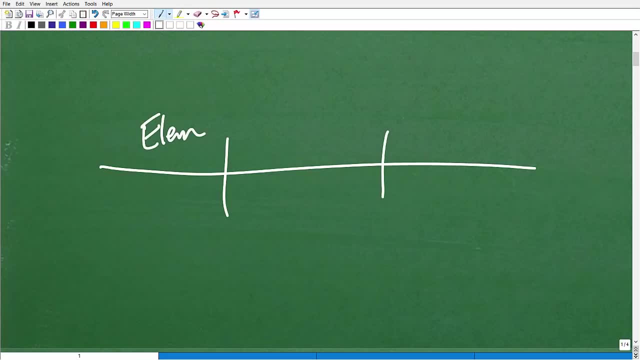 But let's get into calculus. All right, Such a cool math, By the way, if you're curious about ever taking it. So here we have elementary school. All right, Good old elementary school, Such a fun time. Then we have middle school. 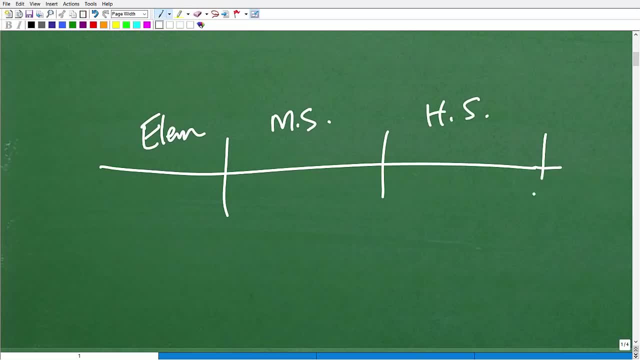 Then we have high school. So in high school you take what? Well, you take algebra one, for the most part. Now, it's Schools are different, Districts are different, But for the most part, these are the courses you need to take in order to take calculus. 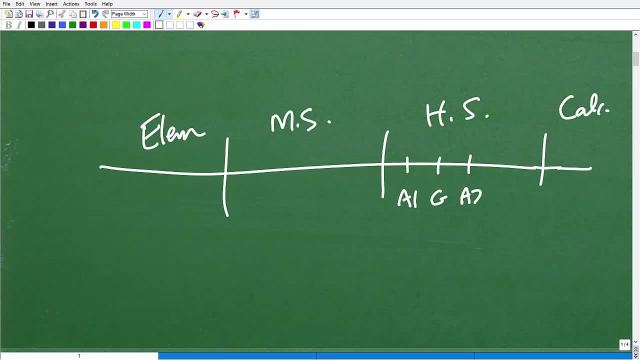 All right, This is what I'm doing here. real quick, You got to take geometry, You have to take algebra two And then you need to take a like a pre-calculus course. Okay, So this is basically advanced algebra two and trigonometry, with some other stuff in it. 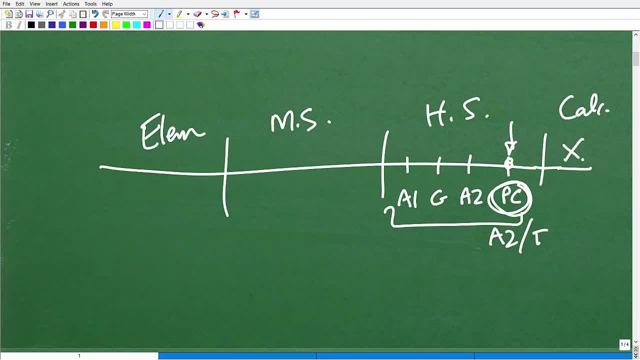 So you got to have all these courses underneath your belt before you take calculus. For the most part, people take calculus in college, Although you could take Calculus as like a senior, like AP calculus in high school, which is the real deal- calculus. 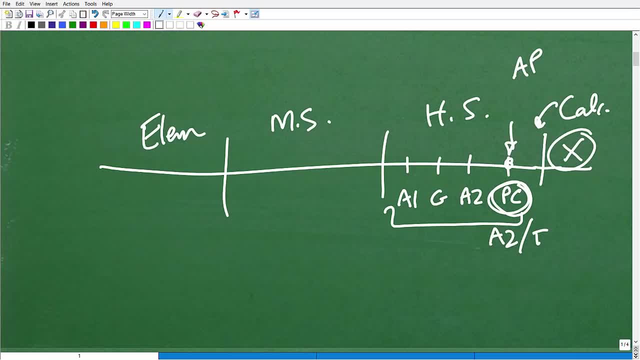 Okay, So there are definitely. you know, math teachers are teaching calculus in high school, But that means you have to be, you know, a math superstar way back in even middle school, All right, So if you're curious about ever taking calculus, this is the course that you need to get yourself up to pre-calculus. 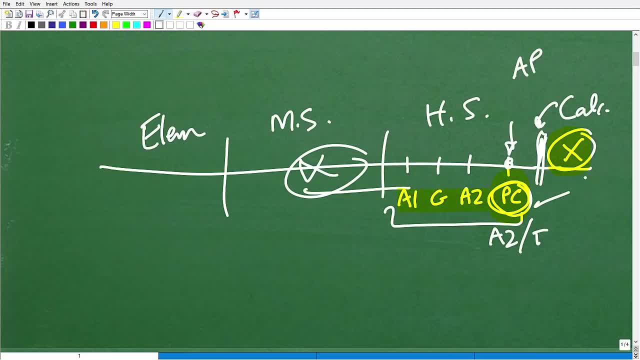 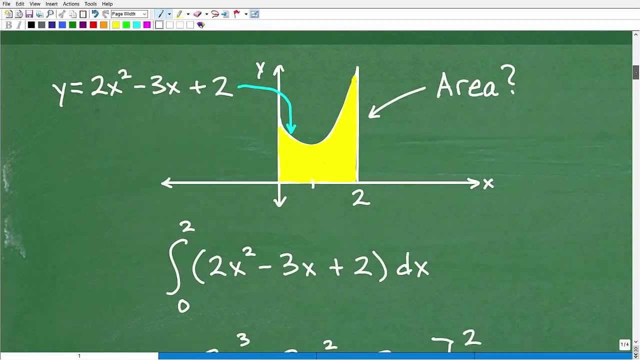 All right, When these are kind of the prerequisites to that course and this course of my pre-calculus course will be ready And It's going to be a matter of weeks. Okay, All right, Let's get to this calculus problem. 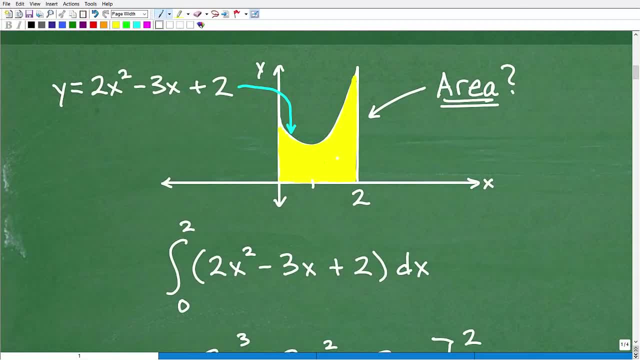 And here it is. So we want to find the area of this crazy looking yellow shape. So In calculus we use these things called functions, and this function, this y, equals two x squared minus three. x plus two is just defining this curve. 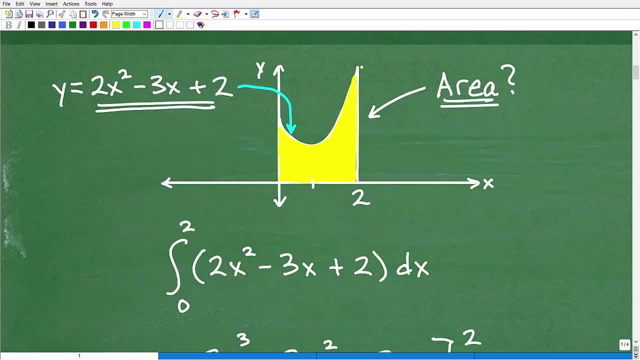 This curve right here, Right, This is the graph of it. Now this actually continues on. Okay, In other words, the curve goes like: so We're only We're only looking at a segment of it. All right, That's all we're doing. 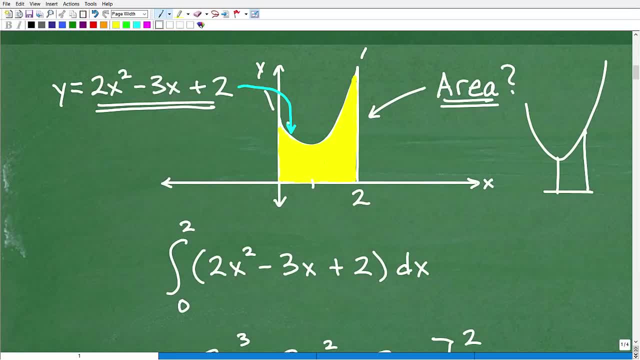 And the segment that we're looking at, this, underneath this yellow, where all this yellow is at, is between zero and two, All right, So we're starting from zero and we're stopping at two, And so this is our yellow curve. That's that's. this is the yellow region. 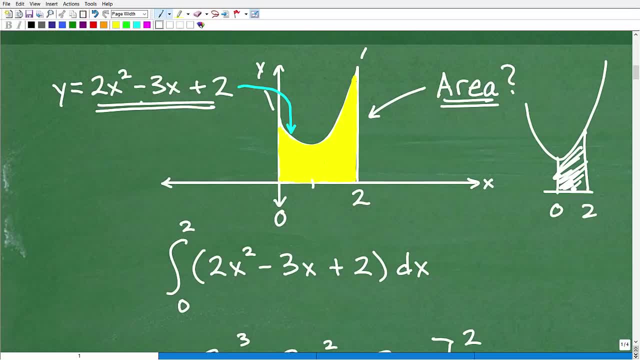 Okay, And it's bounded by this curve. All right, This function. So if I could graph that this way, don't worry about if you don't know how to graph this, Just know that this y equals two x, two x squared minus three. x plus two is a description, a rule on how to graph this shape right here, this curve. 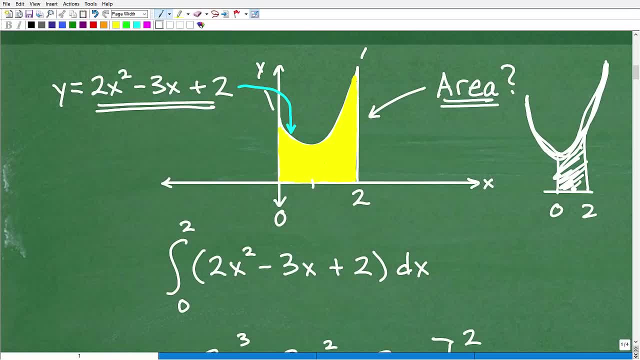 Okay, So in calculus we look at the area underneath the curve And again we're going to go from underneath that curve down to the x axis, and the y axis is going to be kind of its boundaries. Okay, So that's all we're going to be doing. 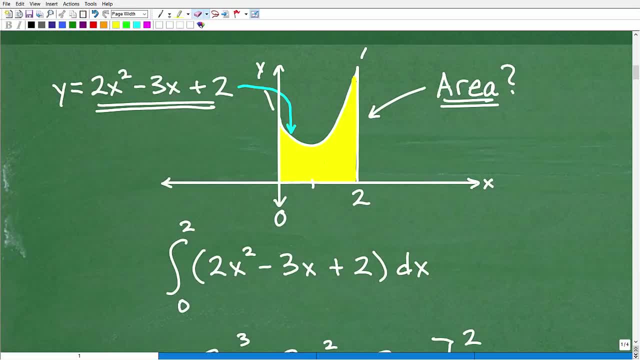 That's the essence, a real basic essence of integration. Now You can see, here I'm using this crazy symbol, right here. This is called the elongated S. And what am I doing here? Well, I want to integrate, All right. 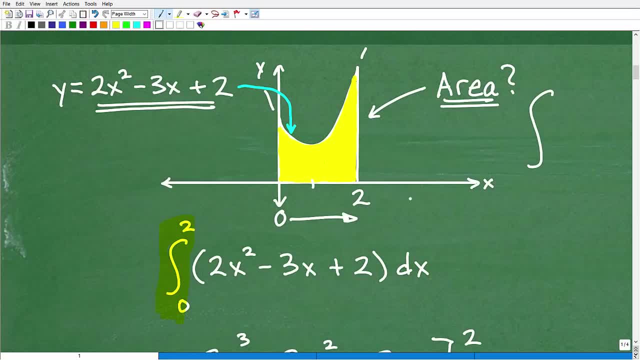 That's what this symbol says, And I want to go from zero to two, So I'm going to start at zero. This bottom number is always your starting point. Okay, So you're going to start from zero and you go all the way to two. 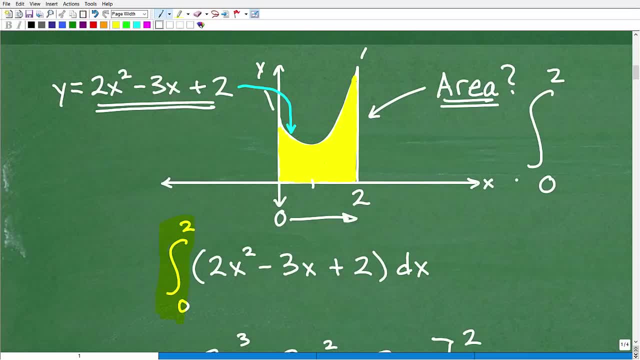 You're going to integrate, Okay, But what does that mean? Well, effectively, that means is you. You can kind of think of it as finding the area underneath this curve from zero to two, zero to two. I got to slow down here because I'm messing up my pronunciation. 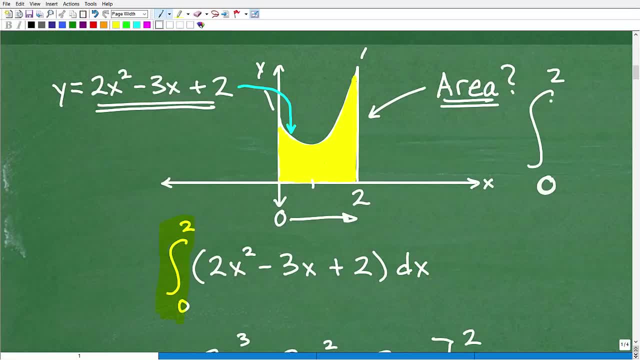 So that's what this symbol is telling us. Hey, start from zero, go to two and give me the area underneath this curve, All right, But what curve You know like? what is the curve here? What is the area? Well, it's this thing. 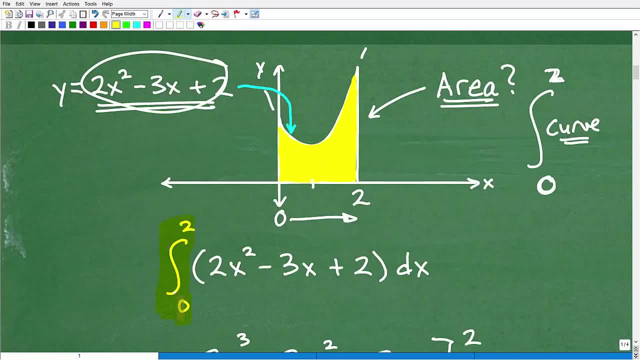 Okay, So that's why I have to write this. Give me the area from zero Zero to two underneath the curve, And this is the curve. This is the description of it. Okay, This little DX. that's just part of the notation that we use. 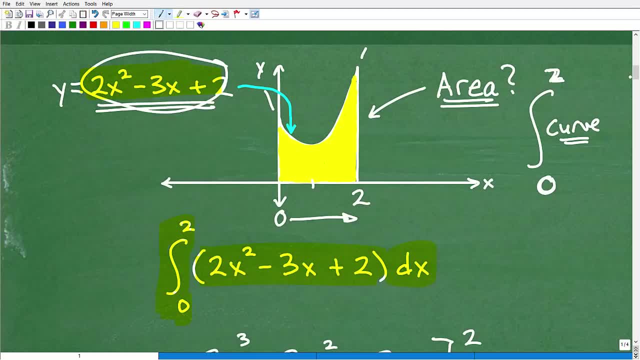 It's, of course, very important, But for our purposes here, you know, it's just part of the notation that we need to use. Okay, So this is the setup. If we can figure this out, we will in fact figure out the area. 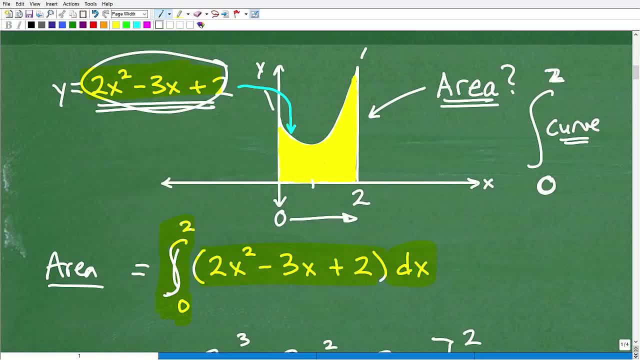 Okay, So that's what we're doing here. We're going to find the area. That's what you kind of think of this symbol is. Hey, give me the area Between zero and two underneath this curve, And this is the curve. 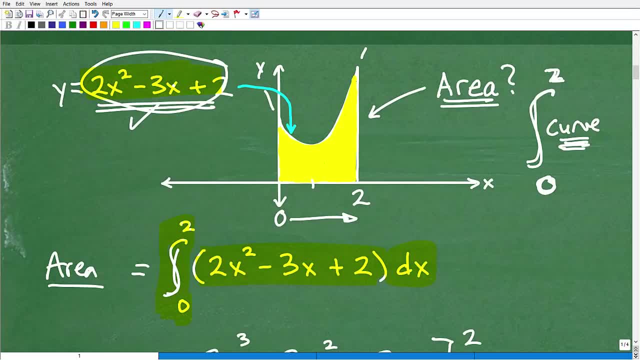 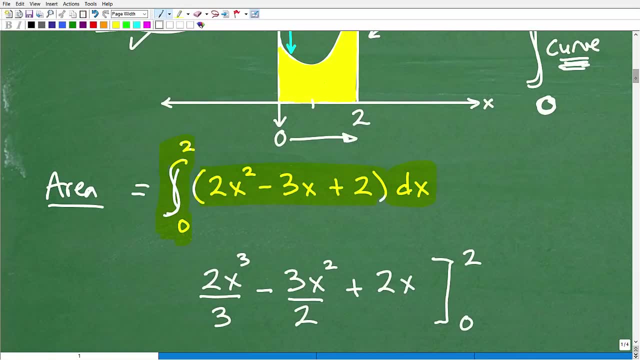 All right. So I mean that's pretty obvious, right? Or pretty straightforward. I mean it's not too scary, hopefully, at this point. Now what we have to do is figure out how to evaluate this, All right. 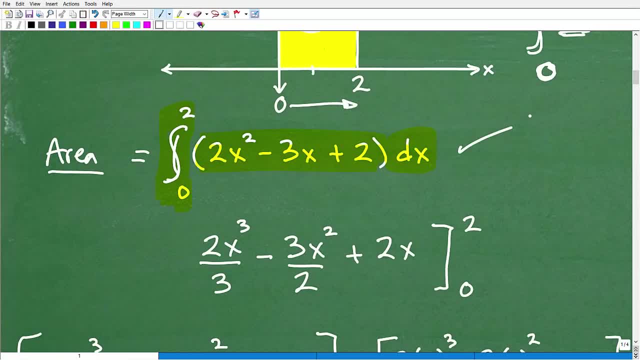 So like: okay, well, I understand this notation, But what do I do with it? Well, we've got to figure out how to evaluate this integral, So here's how this works. Let me go ahead and erase this, All right. 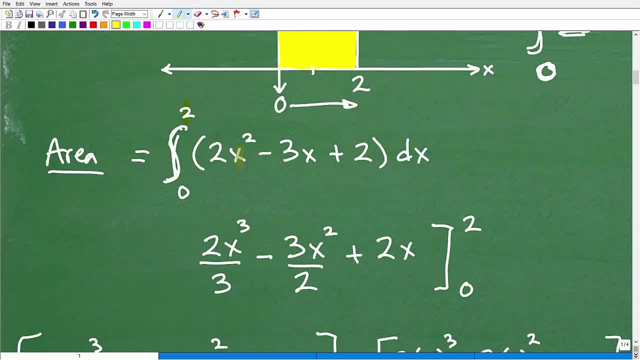 So we fall in calculus like anything. There's just a bunch of rules that we have to follow. So here's what we're going to do to evaluate this. You see this little power two. Okay, Here's what we're going to do. 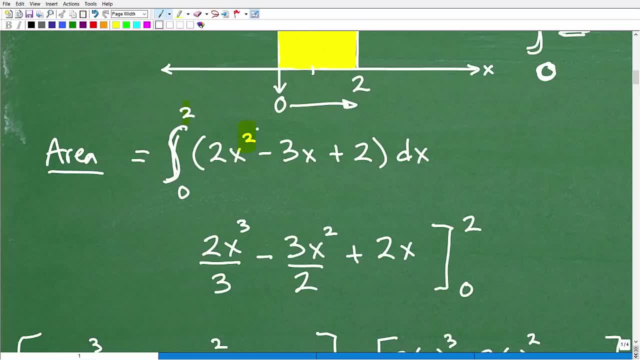 We're going to always add one to the power. So what's two plus one? Well, I think that's three, right? Two plus one is three. So you can see I'm writing this: two X two plus one is three, Okay. 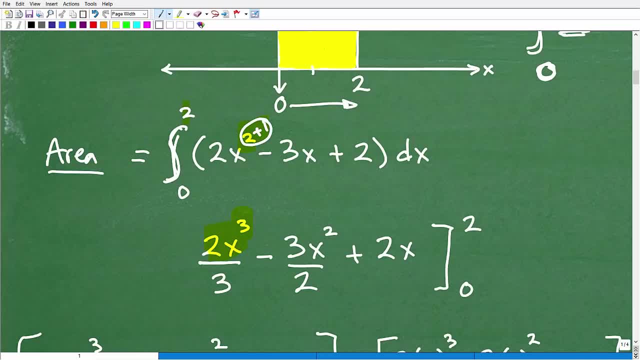 And then, whatever my answer here was, it was three- I'm going to divide by that power. So this three, right there, I'm dividing by it. All right, Do you understand that? Okay? Well, if you do, let's do it again. 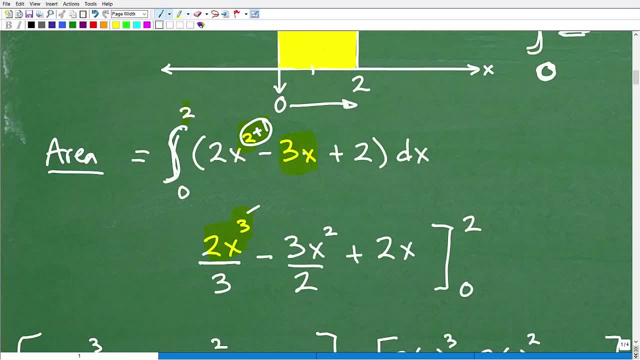 So we have to do the same thing over here. So what is the power? Okay, I have three, X, That's one. So what was the little rule that I did? Well, I have to add one to it. So one plus one is two. 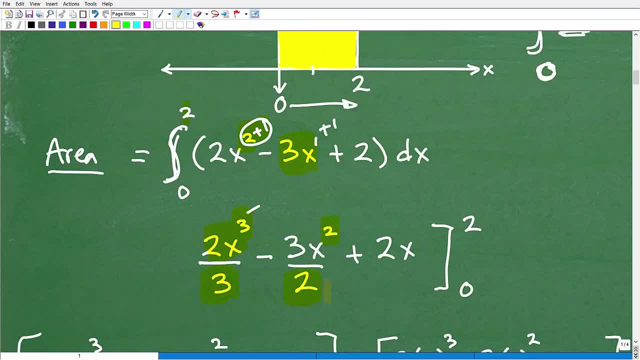 Okay, And then I'm going to divide by the power two. That's what I'm doing here. Okay, Now this two number, In fact this is Two, X to the zero, So anything to the zero. power is one, So two. we're like, well, there's no X's here. 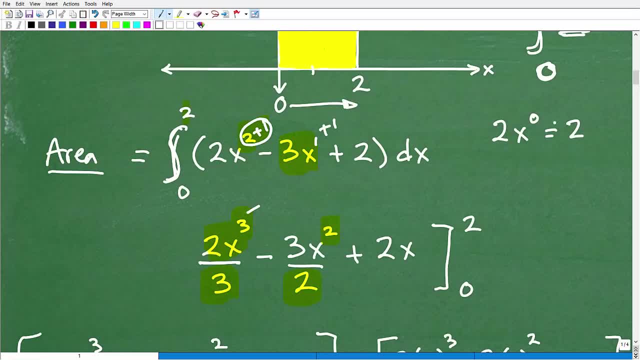 Well, you can think of it as X to the zero power, because anything to the zero power is one, So two you can write: think of as two to the X to the zero power. Okay Now, zero plus one is- excuse me, I'm losing my voice there. 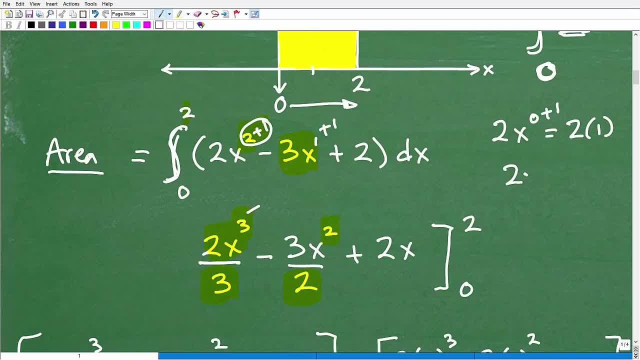 Zero plus one is what It's just one. So that's two X to the first, Or just two X. Okay, So that's what I'm writing like, So, and then I'll divide by one. All right, Now, I'm not going to take that divide by one, because two X divided by one is in fact just going to be two X. 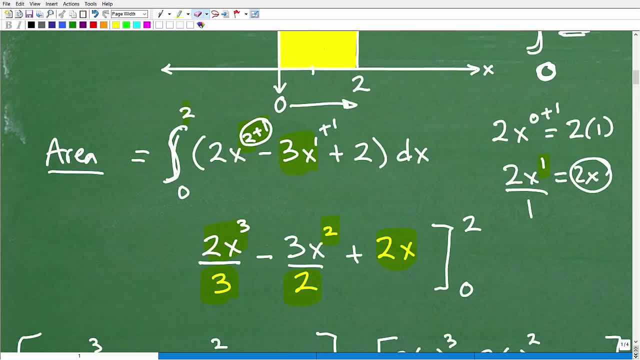 So that's how we get this Okay. So we evaluated the integral and we were able to get it down to this expression And if you're with me so far, like okay, I understand. Well, if you understand, very, very good. 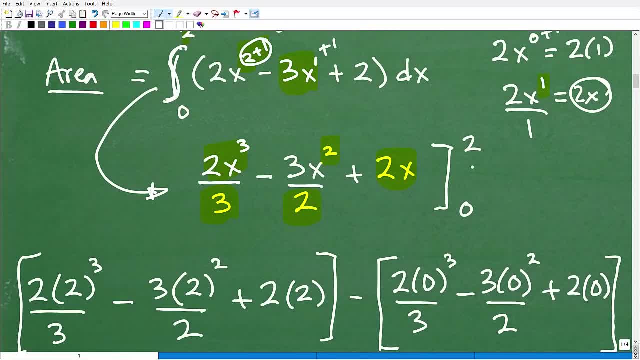 Okay, And now This zero And two, this uh is kind of our little notation- is to say, okay, we still need to evaluate um from zero all the way till two. Okay, Remember, that's underneath our curve. 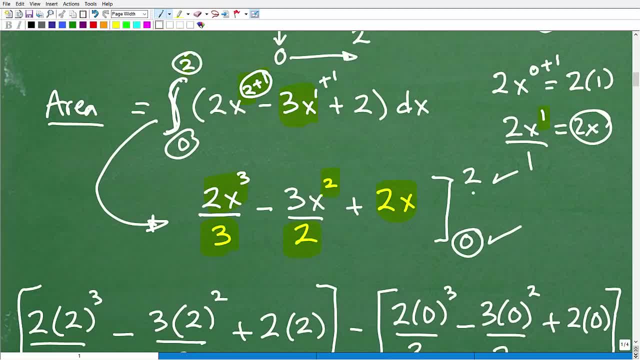 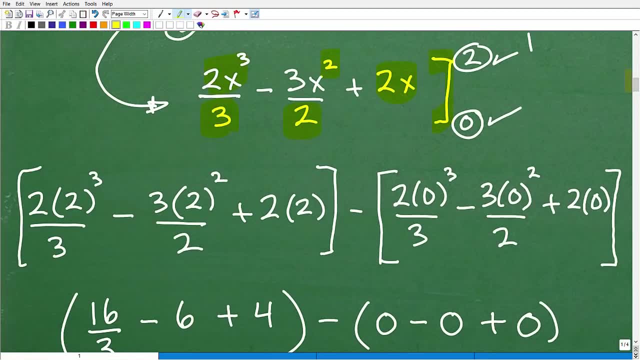 This part of the integral zero to two. we're going to write that little zero to two, just like this. We're going to use this little notation. Now, what does this mean? Well, what we're going to do is the following: 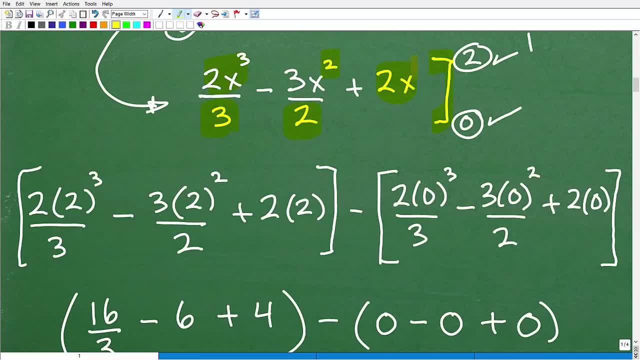 I, of course, I already did it right here. We're going to take this expression right here and we're going to figure out what. Okay, Uh, we're going to calculate some numbers. Okay, The first thing we're going to do is we're going to plug in two, or everywhere. 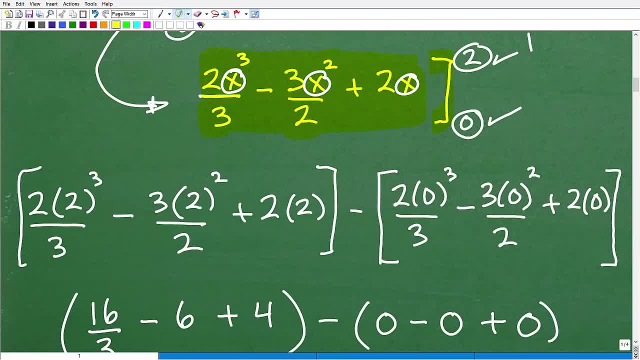 There's an X, I'm going to plug it into. Okay, All right, Then I'm going to do that right here. I'm going to do that first, and then I'm going to subtract: uh, the same thing, But at this time I want to plug in zero. 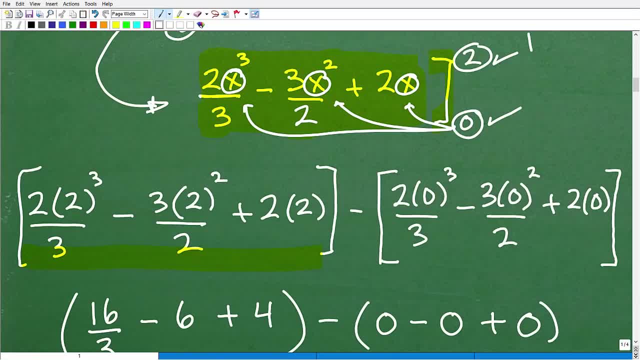 Okay, So I'm going to do this twice. I'm going to figure this thing out when it's two and I'm going to figure this thing out when it's zero. All right, So you can see, this is the setup, right. 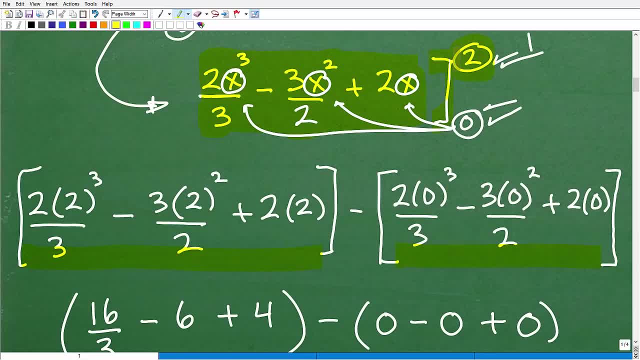 I'll plug it into for the uh, this top number. Okay, First the highest number, I'm going to plug it in, and then I'm going to subtract it away from that lowest number, zero. Okay, Yeah, we're almost done here. 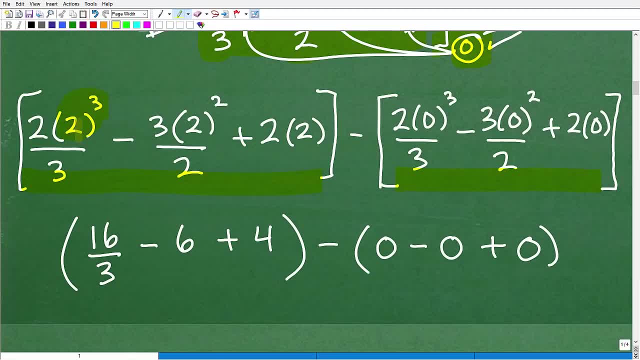 So let's look at this: Uh, two times two to the Q power two. Uh, that's two times two times two, That's eight times two, That's 16 thirds. This will be four. Okay, Two squared is four times three. 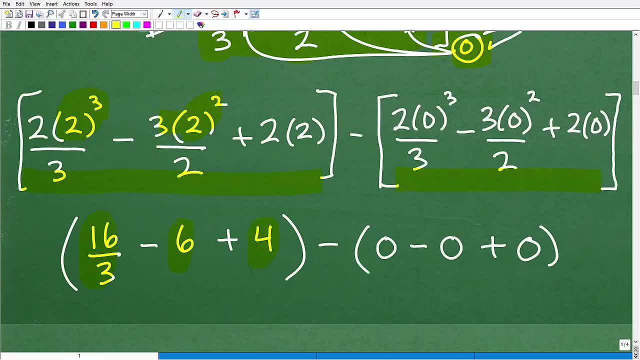 Uh, that is: 12 divided by two is six, and two times two is four. And then here I have all these Zero That's going to make this whole entire thing zero, because I'm going to end up with zero, zeros in each one of these little terms. 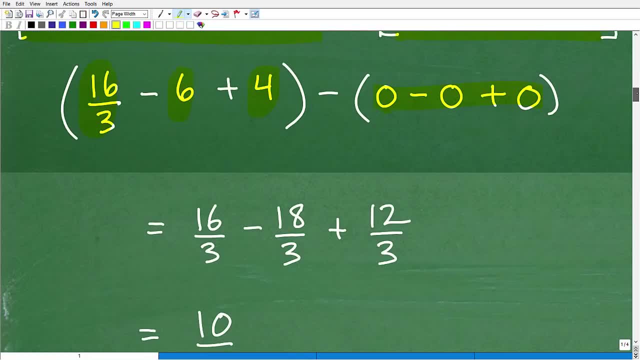 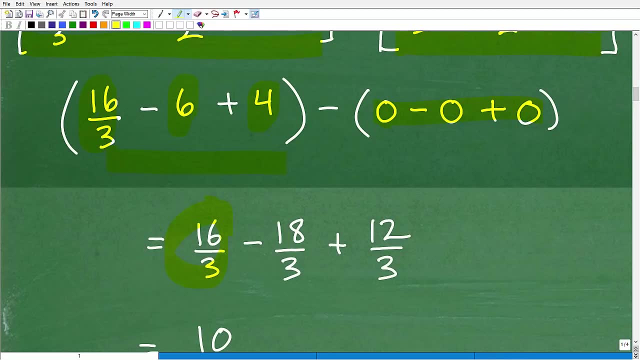 So that's a zero. So all we have to do is figure this out right here and we will have solved the problem. Okay, So 16 thirds six is the same thing as 18 thirds. Four is the same thing as 12 thirds. 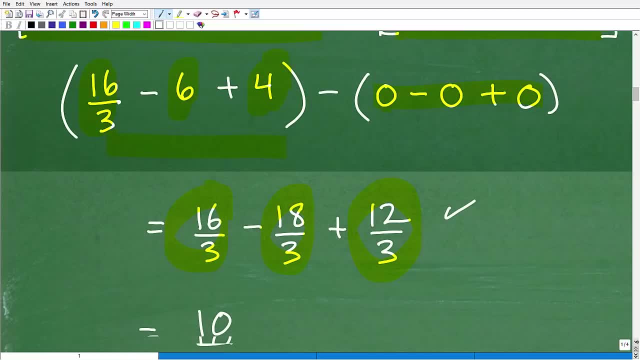 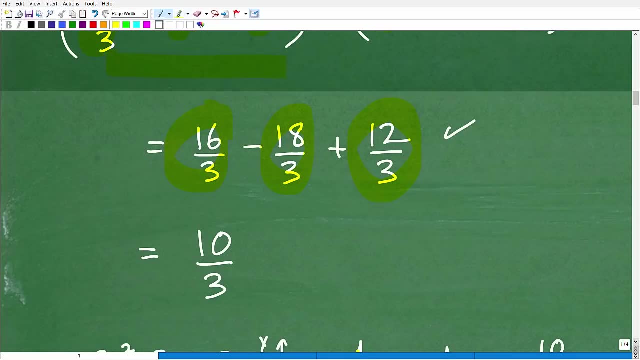 I know that all of you are excellent in your fractions. By the way, if you're struggling with fractions, I have tons of videos in my pre-outro playlist. Uh, that can uh really show you the secret, uh, to being excellent at fractions. 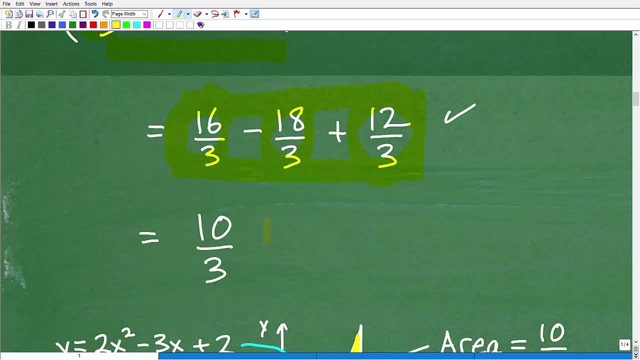 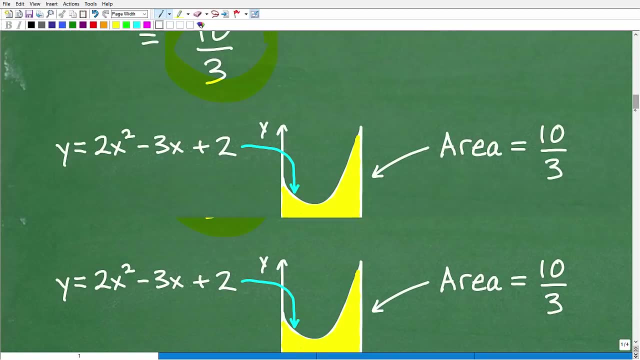 All right. So would you all this little um addition and subtraction of fractions, you get 10 third. All right, 10 thirds. And what does that mean? Well, that is in fact the area we are done, Okay. 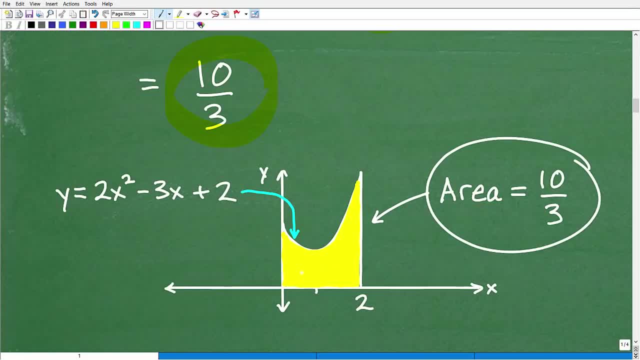 We have calculated the area, uh, of this little crazy yellow section right here bounded by this function, from zero to two. The area is 10 thirds and that's it. That is a demonstration of Integration in calculus and uh calculus, for the most part, uh, basic, uh, basic, first semester calculus course or first year calculus course, is broken up. 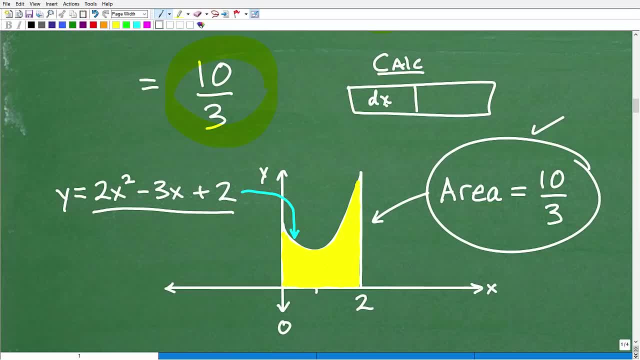 Um, uh, one half you're kind of studying this thing called uh, derivatives, And then the other half you're studying this thing that we just did here called integration. Okay, And uh, integration. one of its main primary applications is finding the area underneath the curve. 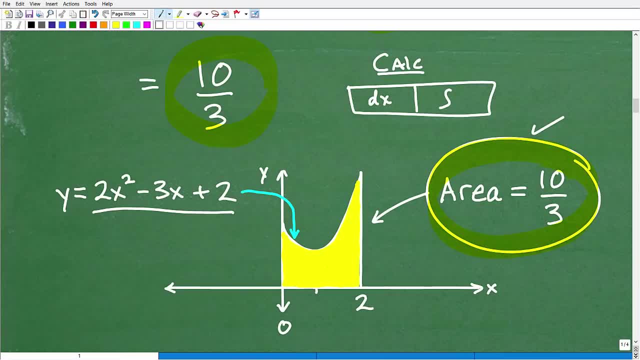 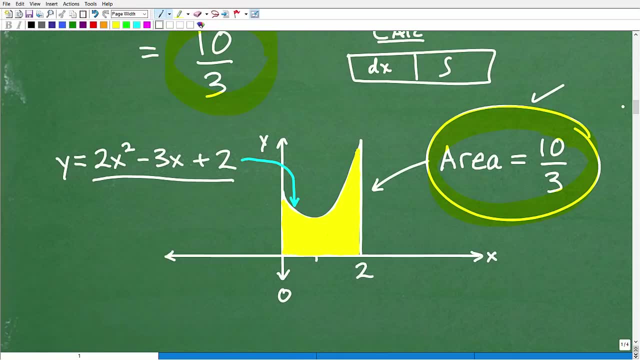 And we just did this. Okay, Now, hopefully This was Uh relatively understandable to uh most of you out there, but maybe a lot of you were saying like I completely understood, This was awesome. If that's the case, that's excellent. 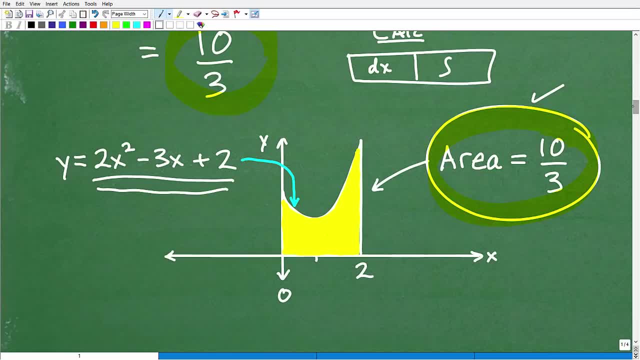 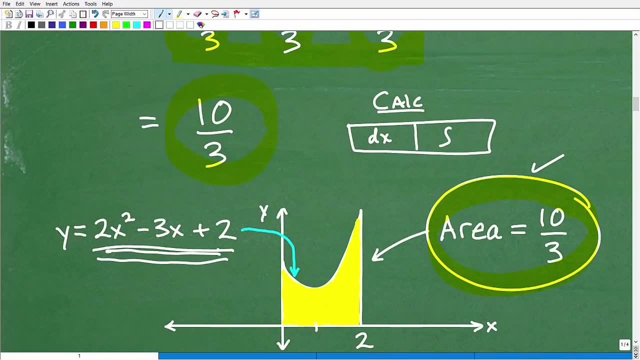 Then I did my job Okay, But maybe you're a little bit shaky on the math or maybe I went a little bit too fast on uh, you know, maybe you're like I don't really quite understand these functions. Listen, if this is none, of this is beyond what you can do. 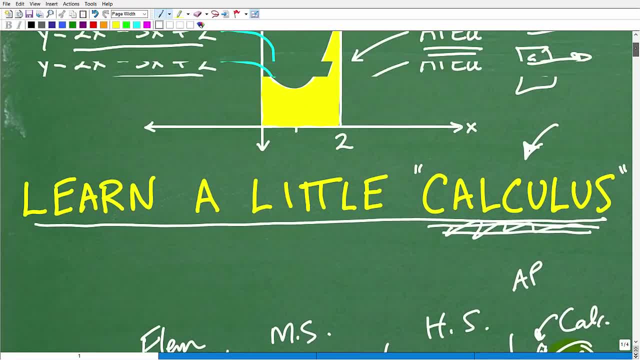 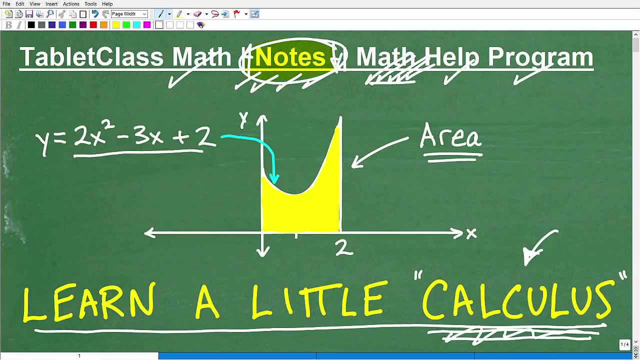 Okay, Uh, I'm telling you right now: if you want to take calculus, you can definitely take it and learn it. I don't care If you failed out of elementary school. all right, you can do far more than you think you can do now. 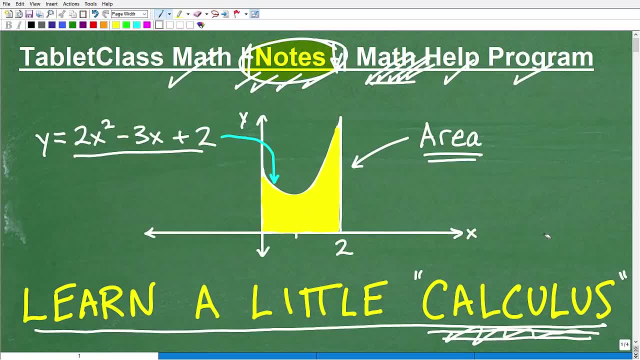 Do you need to have, um, you know, uh, a good prerequisite, good foundational knowledge and stuff to actually take calculus? Yes, you do. Now, if some of you are actually in calculus and having a tough time, it's likely because your foundation, uh, wasn't strong enough. 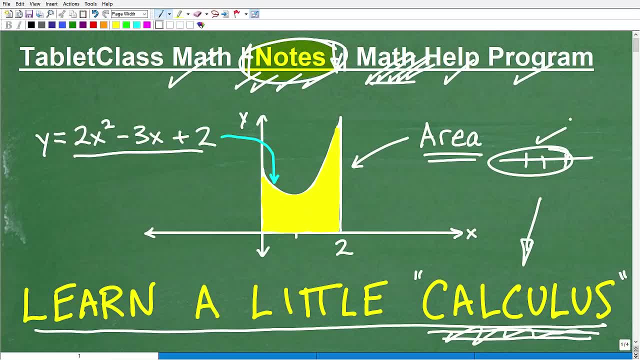 Okay, You didn't have- uh, maybe you did mediocre in high school- of a mathematics. You can correct that, Okay, Okay, Okay, Okay, If you're having a tough time in calculus, it's: uh well, it's one of three things. 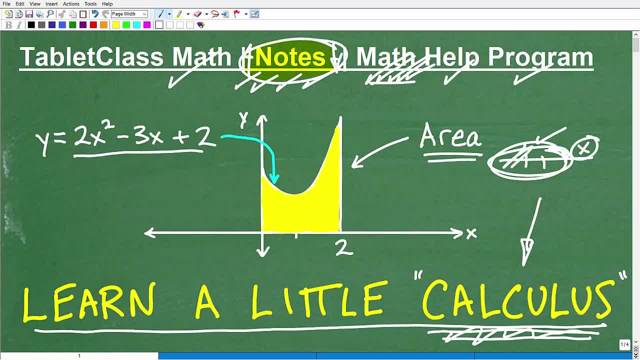 One, I would say that your foundation was not strong enough, which means you're going to have to go back and, uh, strengthen your foundation. Okay, That's number one. Number two: um, you're not working hard enough. you know, maybe you're taking notes. 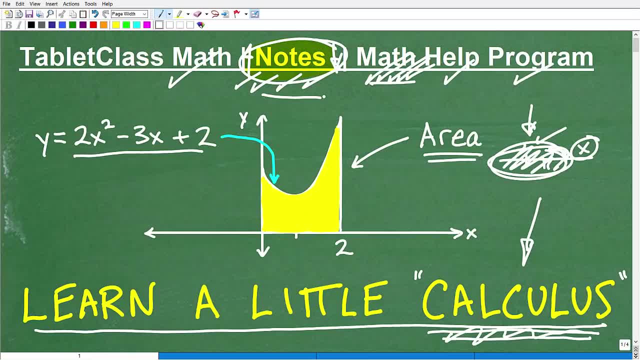 You're like: I'm doing my best. Listen I'm talking about. you're going to have to go above and beyond. You're going to see your teacher. You're going to have to do anything and everything to help yourself, because it's a difficult course. 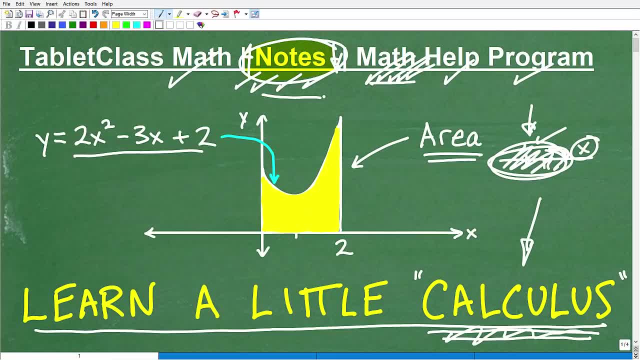 Right. So, uh, that's that's the second thing I would say is that you're not working hard enough, Okay. And the third thing is I think that, um, you know, you possibly could have, uh, uh, been. 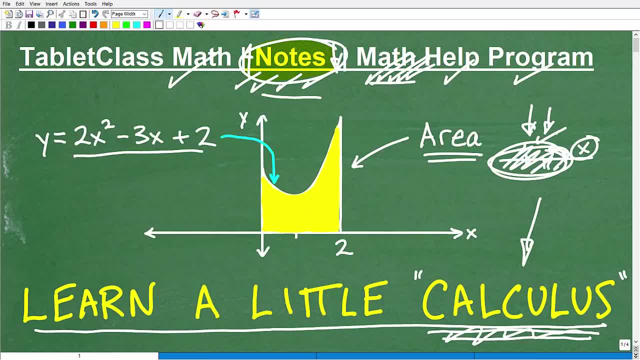 placed into the wrong course, Right? So if you did take pre-calculus, uh, then you should be ready for calculus. Now, um, if you haven't taken pre-calculus and maybe took something and your college says, oh no, you, you can place into calculus. 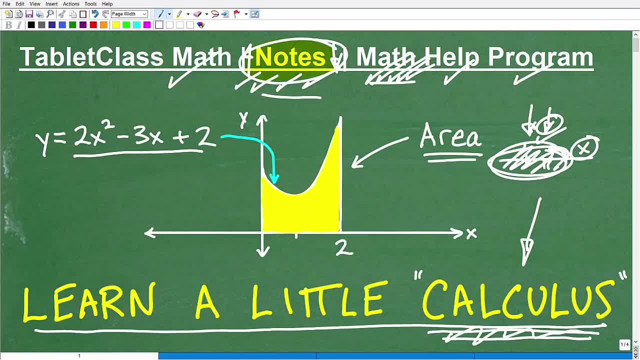 Well, you know, you might want to, um, you know, discuss that with your, uh, your, your university or college or wherever you're, you're your teacher, and be like: Hey, do you really think I'm ready for calculus? 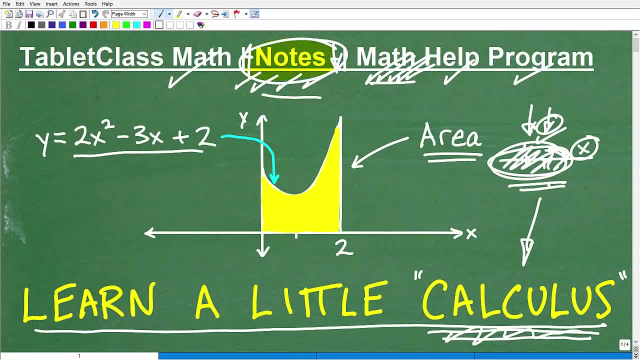 You may not, In fact, you might need to take another course before you're in fact ready for it. But listen, the bottom line is is a ton of people, millions of people, have taken calculus successfully and uh, trust me, you can uh successfully learn this, but it is work and